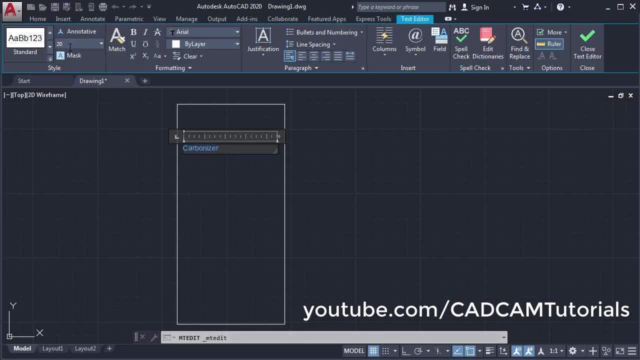 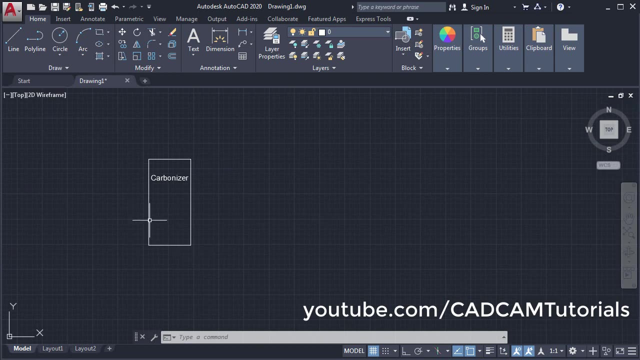 20 is also smaller. again, double click on it, select it and make it 45, enter. We can still increase it. suppose we will make it 55, enter. click outside, Then zoom minus, Then we will copy this block here. for that, click on copy. 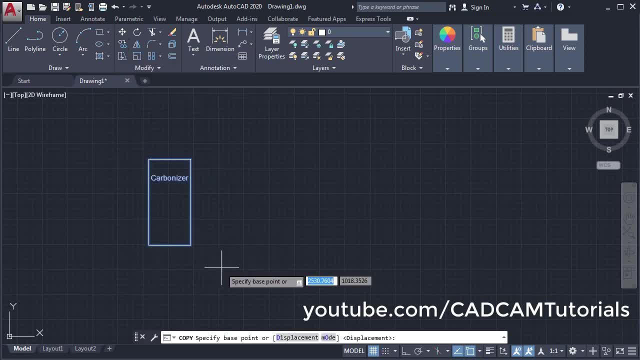 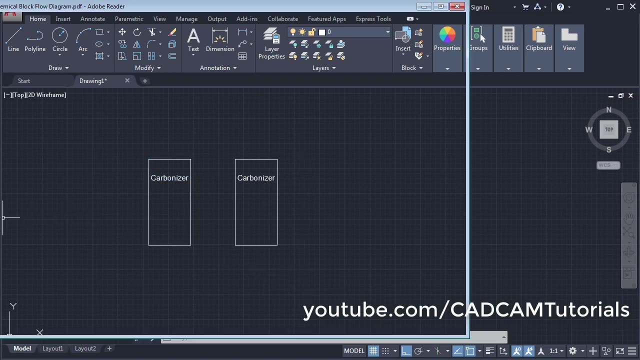 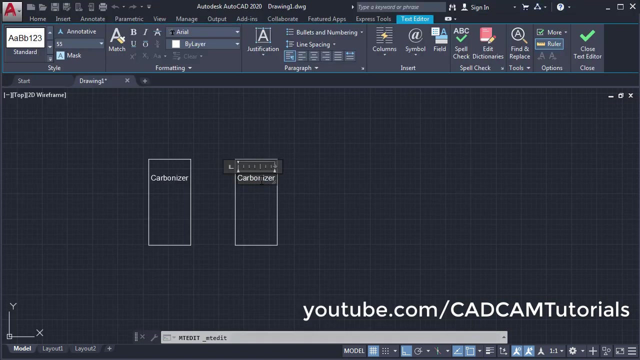 Select this object, enter. specify base point. I will click here, then make ortho on for straight moments. take your cursor on this side and click and enter. Then this is primary fractionator. Just double click Then select it and type primary. 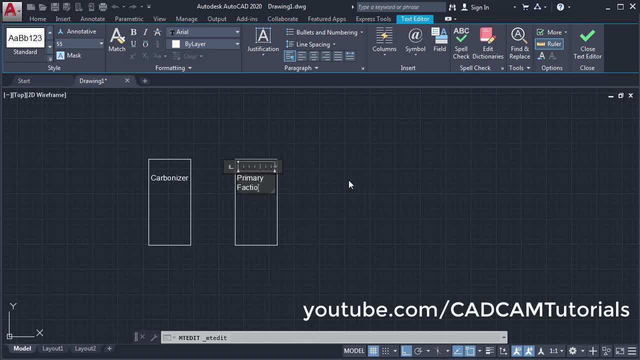 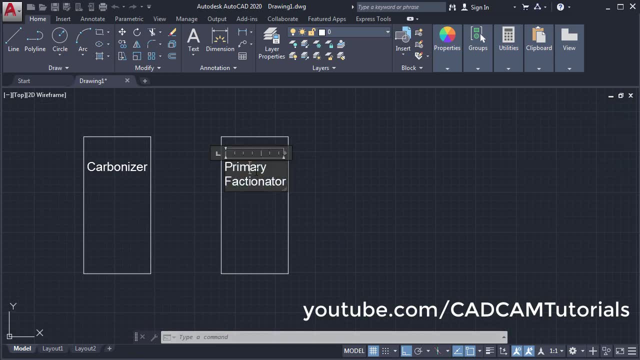 Enter, Enter, Enter, Enter, Enter and click outside. Then we can align it centrally. just double click on it, Select this text And click here on center and click outside, And if you want to adjust the position, you can use the move command. 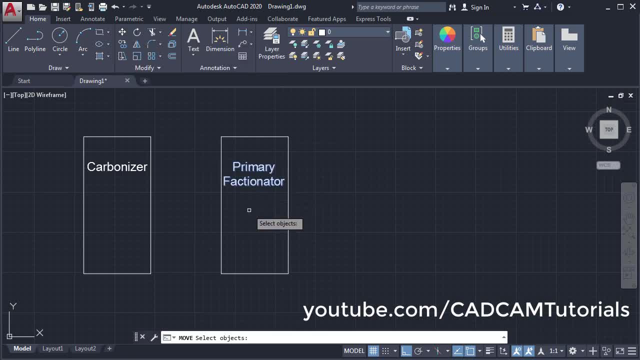 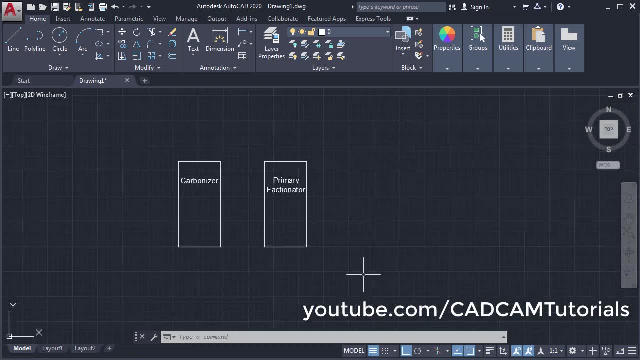 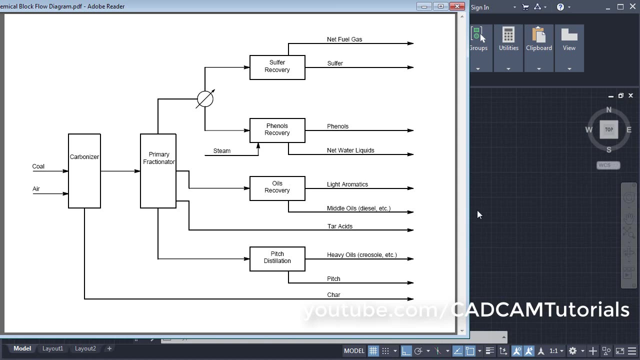 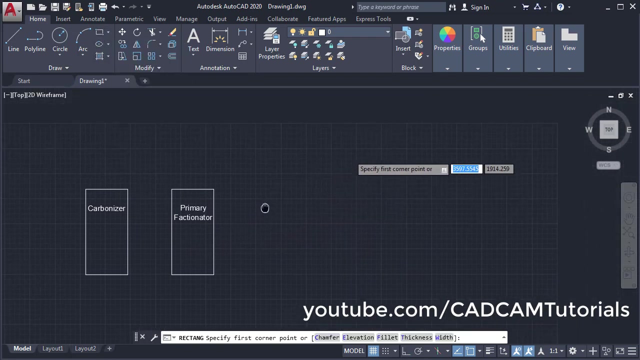 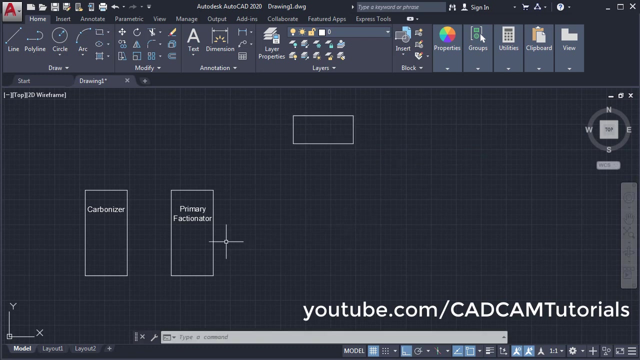 Click on move. Select this text, enter, Click base point And adjust the position and click and zoom minus. then we will create these four blocks. for that again, click on rectangle, pan it below, specify first point, take your cursor on this side and click, then we will copy this text. click on. 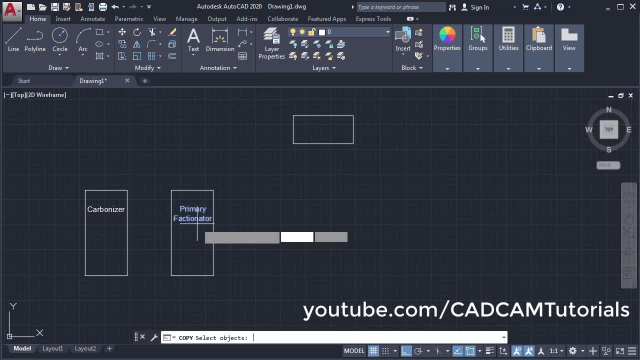 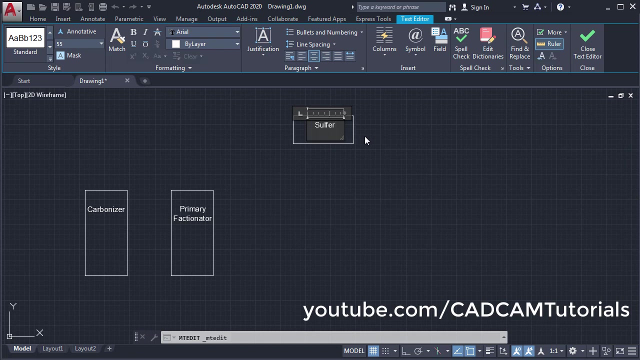 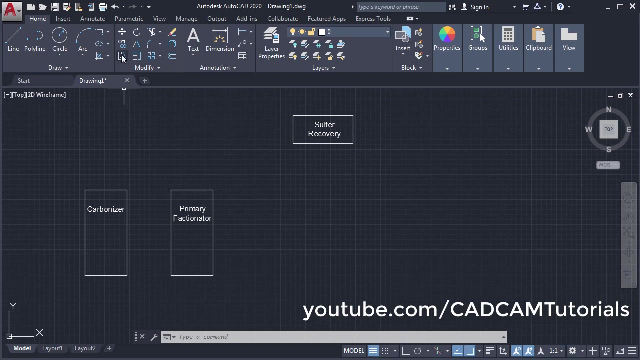 copy. select this text: enter. specify base point. make ortho off and click here. enter. then this is sulfur recovery. just double click and type sulfur, enter recovery. click outside. then we want four copies of this. click on copy. select this object. enter. specify base point. for straight moments, click on. 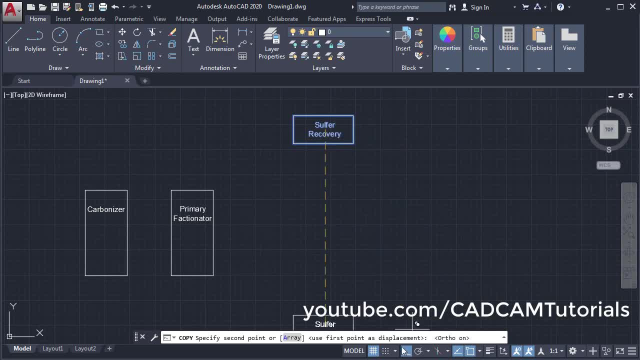 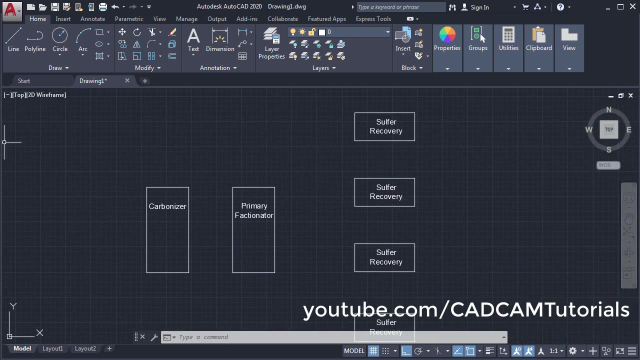 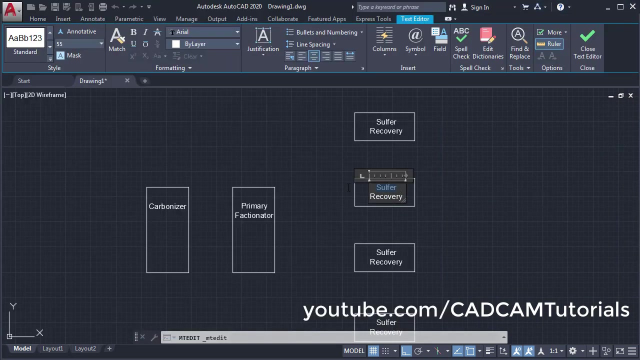 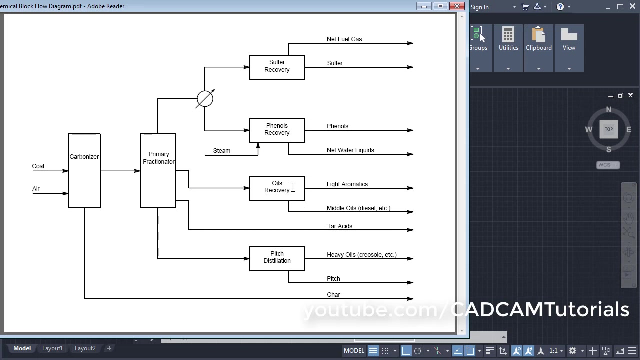 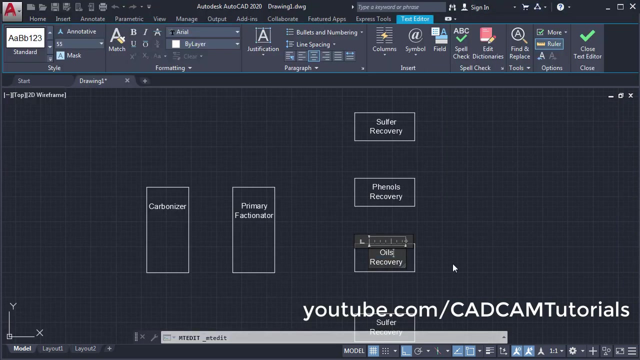 ortho mode. make it on. when it is on, it is shown in blue color. then take your cursor below and click four times. pan it enter than this is phenol recovery. just double click and write their phenols, then oils and peached distillation. you, you. 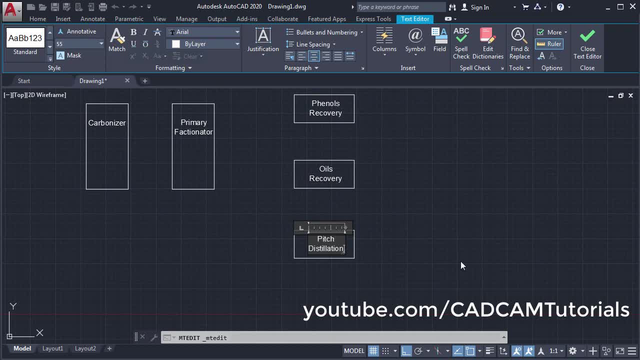 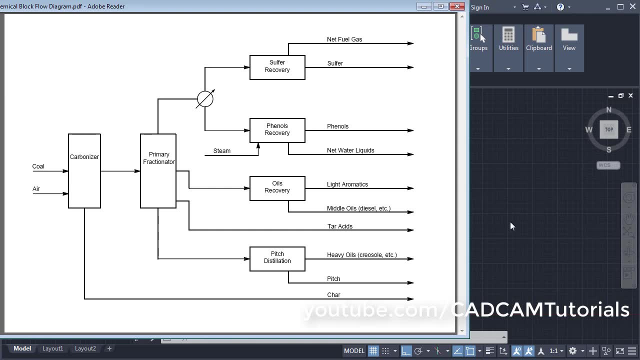 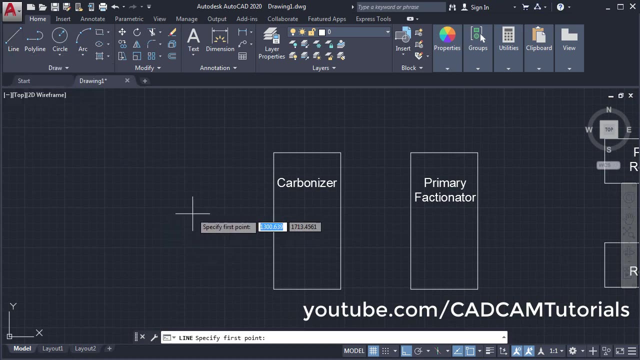 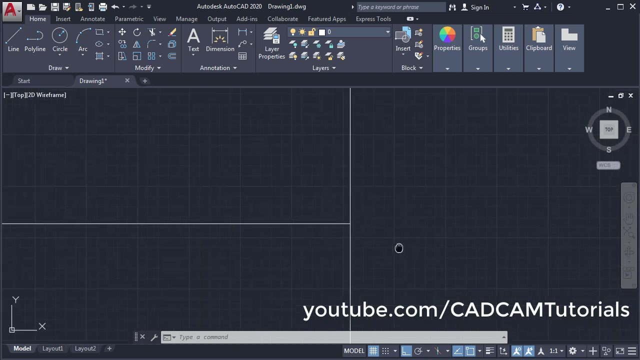 enter you, you, Then we will create this line and this arrow. Click on line, specify first point: take your cursor on the right side, take your cursor to this midpoint, take it above and click and press enter. Then zoom it. then we have to create one arrow here. 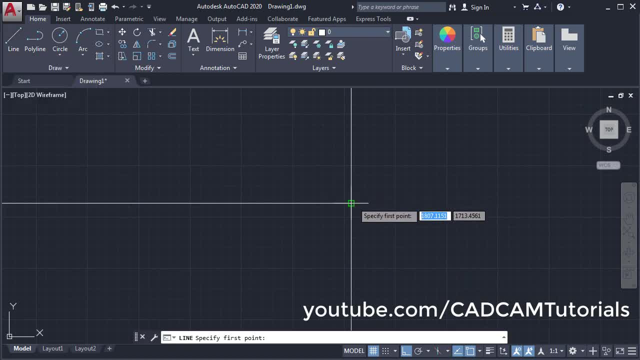 For that again. click on line. specify first point here. make ortho of take your cursor in this direction and click enter, Then we will mirror this line. Click on mirror. select this line enter. specify first point of mirror line click. 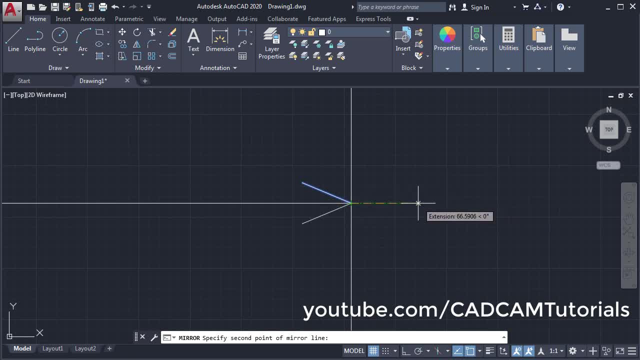 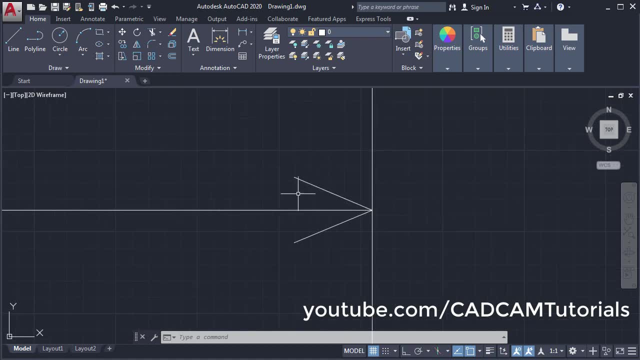 on this end point. Take your cursor on this side. Ensure that your line is straight. Click and erase all subjects. no, Then we will create one arc here For that. click on three point arc. specify first point. Then take your cursor to this end point and track that point. don't click there. take. 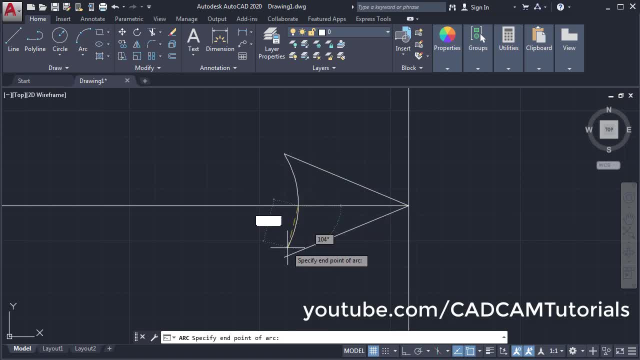 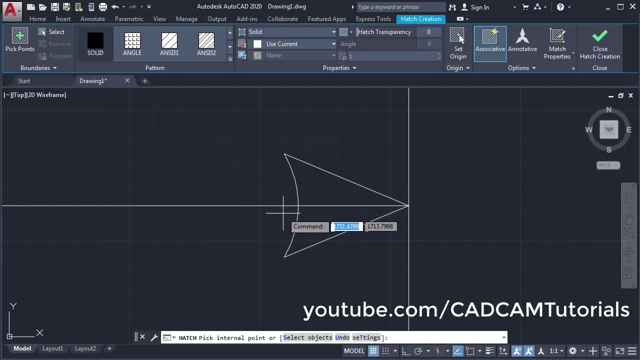 it away and click here, Then click on this end point. Okay, Then, to fill this arrow, we will use hatch command. Click on hatch, then click on solid, then click inside this arrow, Then click on close hatch creation zoom minus. 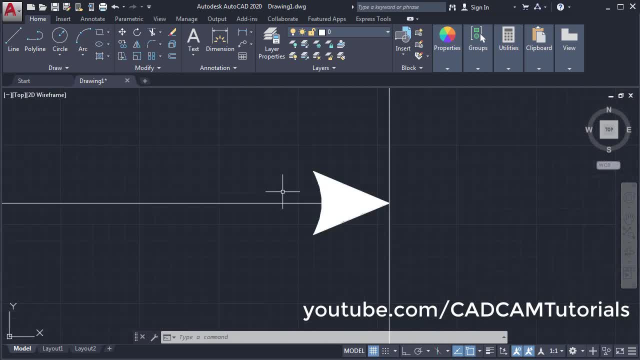 So we will adjust this arrow, we will just stretch it outside. Click on stretch. Click on the right side in the empty space. take your cursor on the left side and click Enter and specify base point. take your cursor on this side, make ortho on and click. 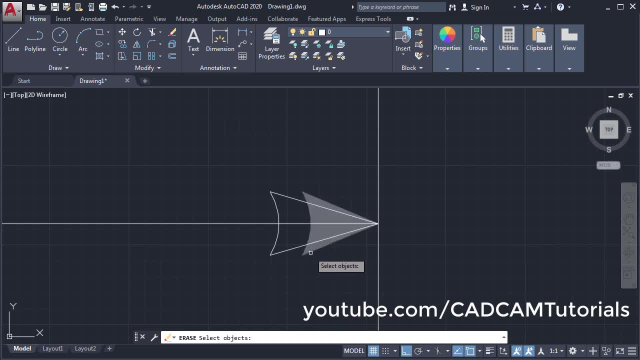 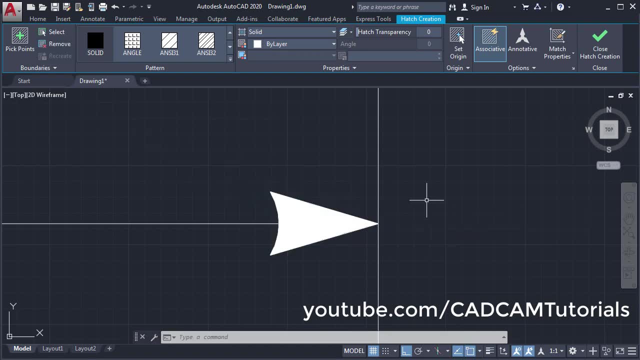 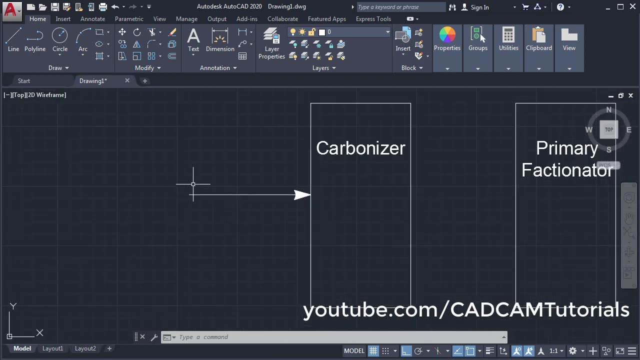 And erase this hatch E enter. select this hatch enter. we will again apply hatch. Click on hatch and click inside this arrow enter And zoom minus. Now this arrow is looking proper. Then we will need one text here. we will copy this: 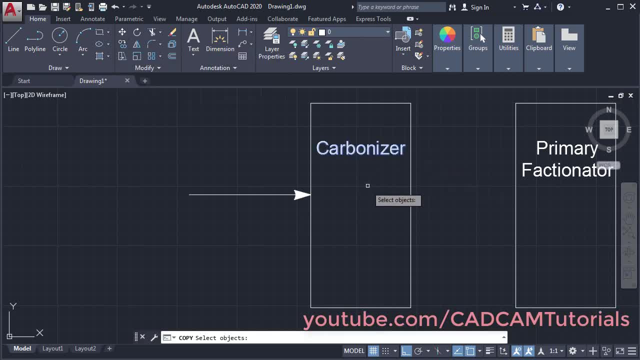 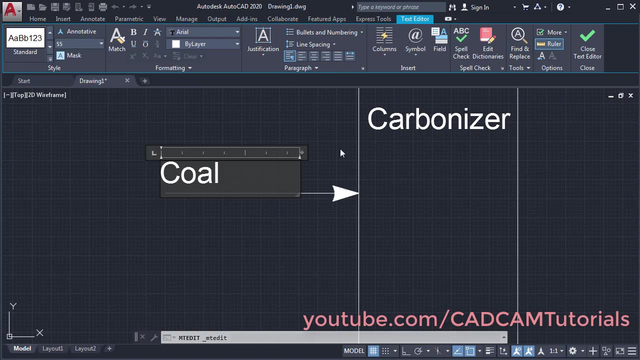 Click on copy, select this text, enter. click here for base point. make ortho of click here, enter Then double click and right there, cool. Then what we will do is we are going to create a base point here. 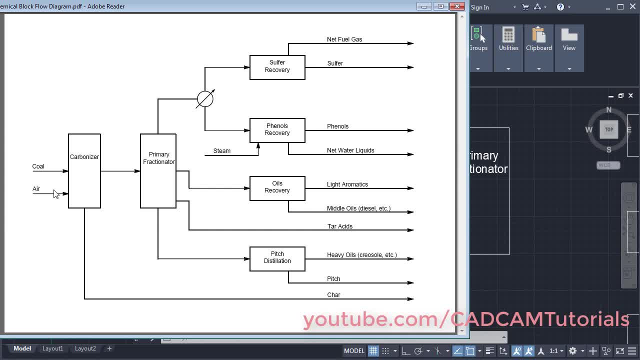 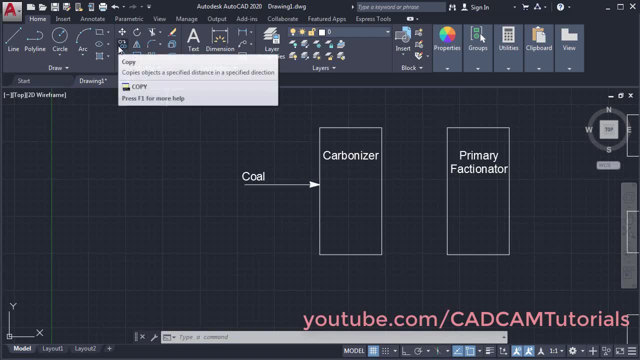 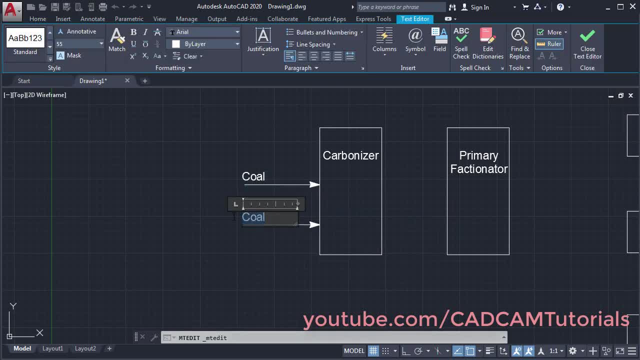 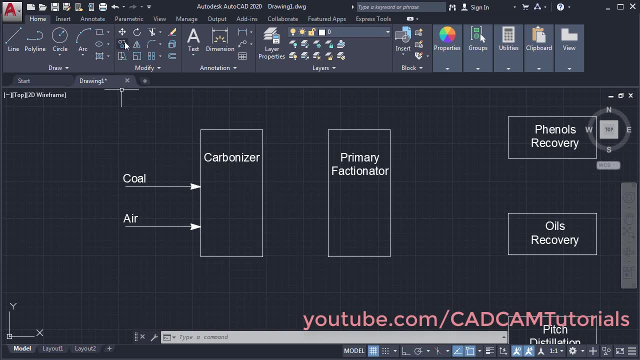 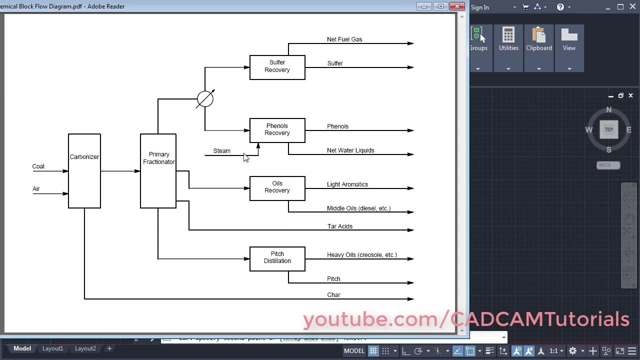 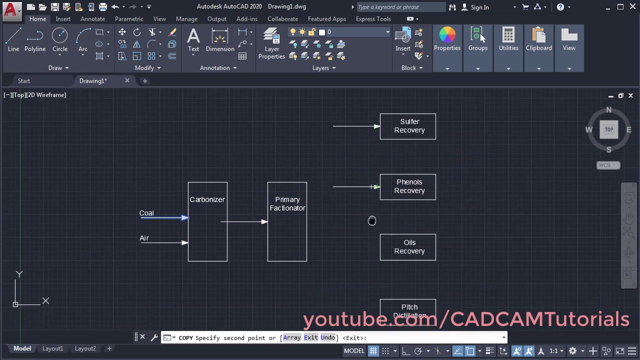 and click enter And make it air. Then we will need arrow here again copy: Select this object, Enter, specify base points here and click on this midpoint. Then we will also need arrows for all of them. So we will just copy here also in this midpoints. 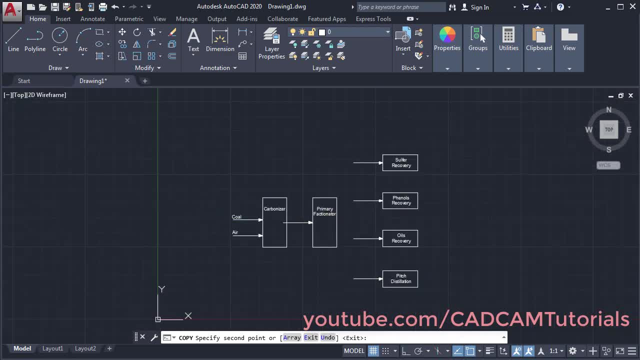 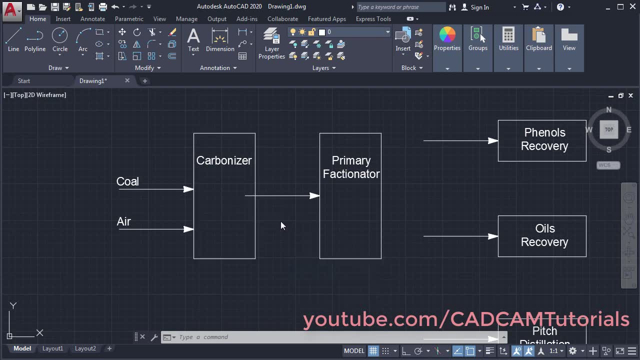 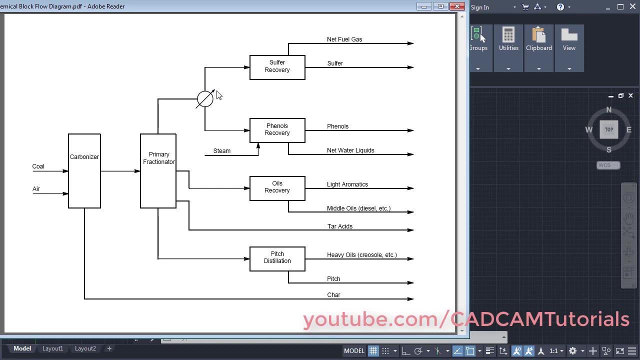 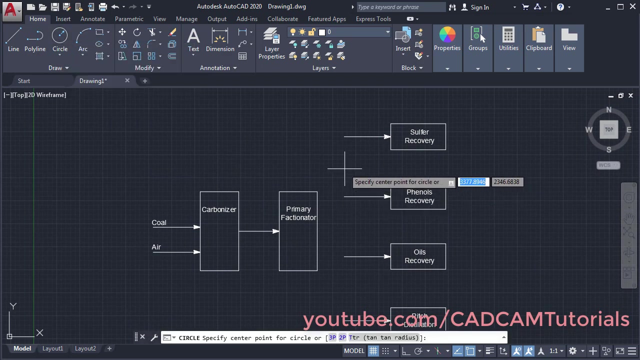 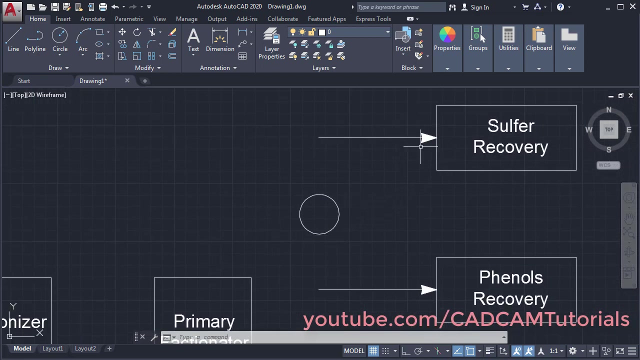 Enter, Then we will trim this For trim type TR: enter, alt And paste, enter and click and enter. the next is this circle and this arrow. click on circle, specify center point. take your cursor away and click. then we need one arrow. we will use this arrow. click on copy. select this arrow, enter. 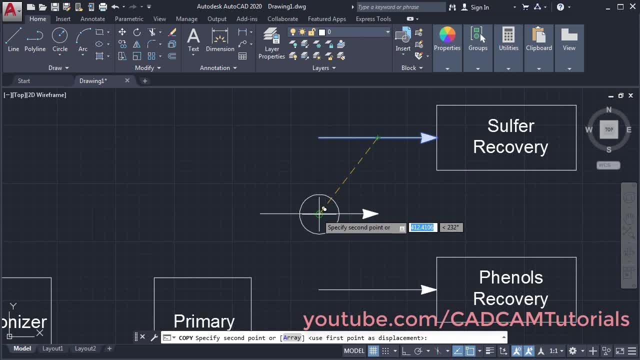 click on this midpoint and click on this center point. enter. then we will rotate this arrow. click on rotate. select this arrow. enter this point will be this midpoint. then give the rotation angle of 45 degree. enter. then we will have to reduce the scale of this arrow. for that, click on scale. select this object- enter. 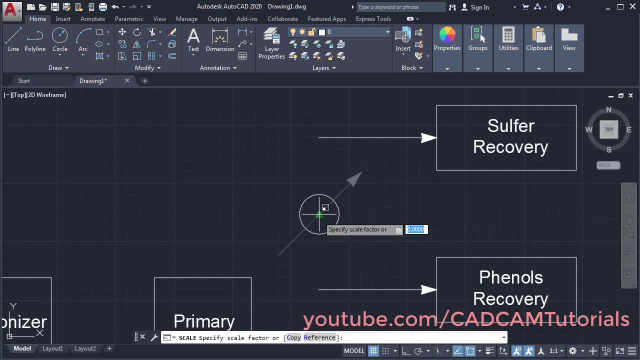 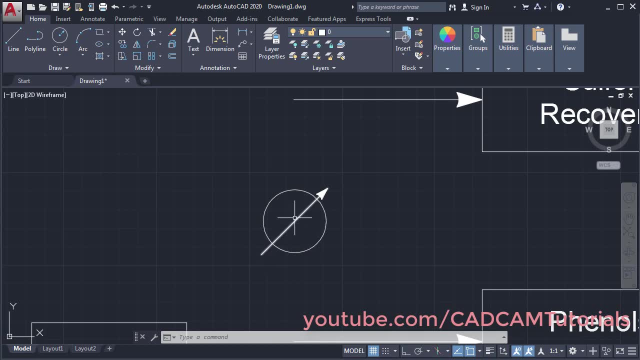 specify base point at this midpoint, then specify the scale of 0.5. enter. now it is looking very small. we will increase its size again. click on scale, select this object, enter. specify base point and make it 1.3. enter- now it is looking proper. 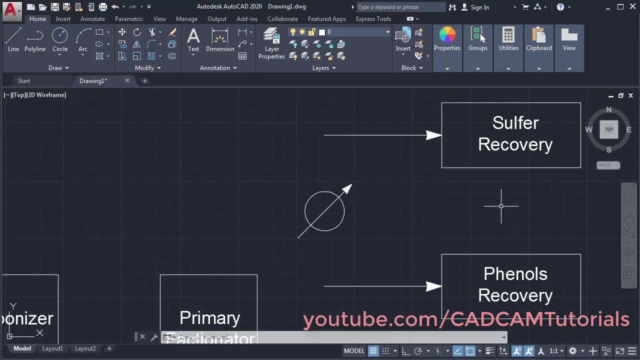 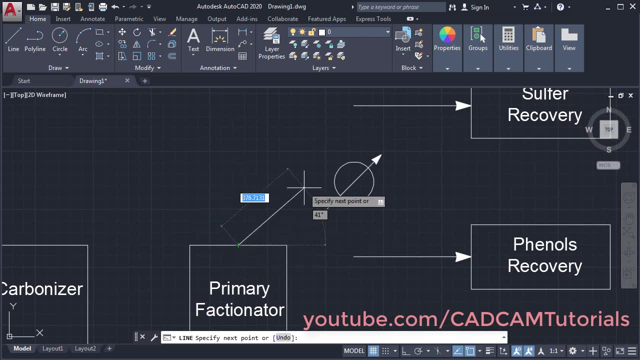 then we will create this line and noisy. click on line, move it to the finger Xiao, drag and drag to this rim. move it to this frente. we will create these lines. repeat now, move it to this rim. press enter. choking, alright, ok, on this intersection point. enter, enter, click on this end and click on this. 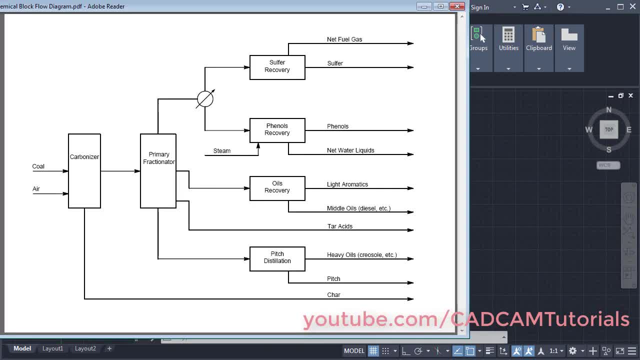 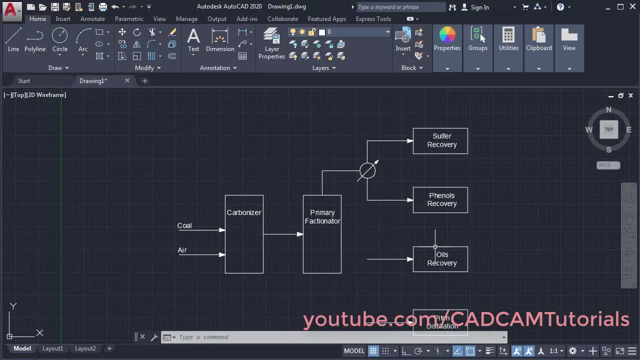 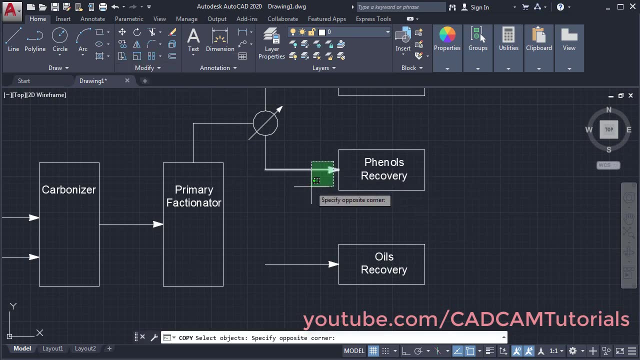 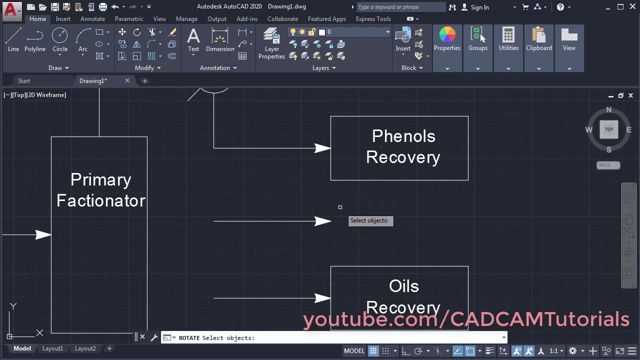 intersection: enter. so this is almost ready. then we need one arrow for this team. we will again copy this arrow. click on copy. select this object. enter. specify base point. take it below and click and enter. then we need to rotate this arrow for that. click on rotate. select this object. enter. specify base. 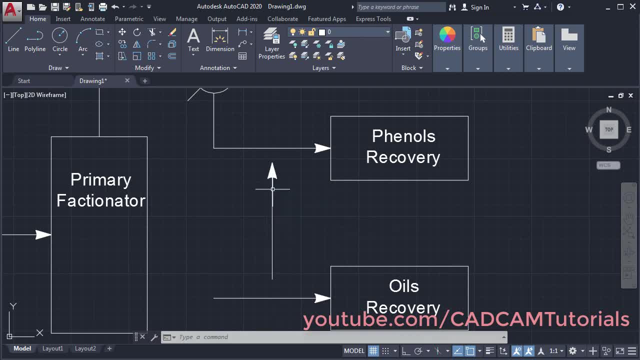 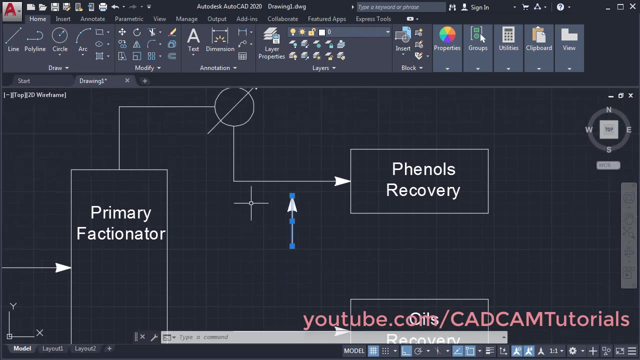 point. take your cursor above and click then to reduce the size of this line. click on this line. click on this blue grid. take your cursor above, make ortho on and click, then we will move this arrow. press escape. click on move. select this object. enter. click on this end point. make ortho off. 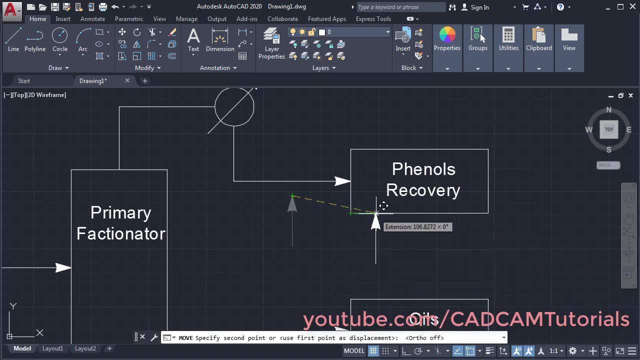 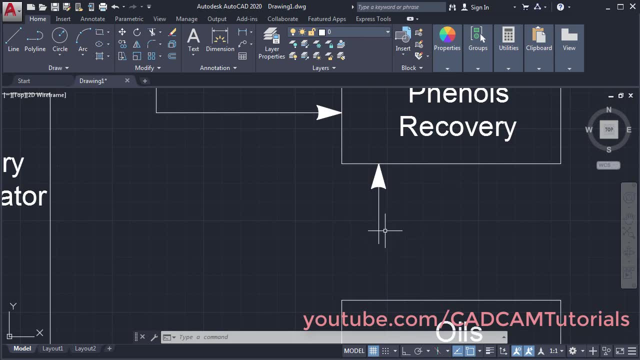 then take your cursor to this end point, take it away. it will track it. click, then we will follow the steps in this video. further reduce the size of this line. click on it. click on this blue grip, take it above and click, then we will create one horizontal line. click on line click. 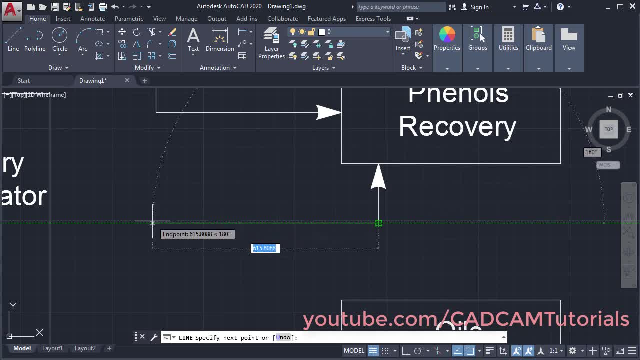 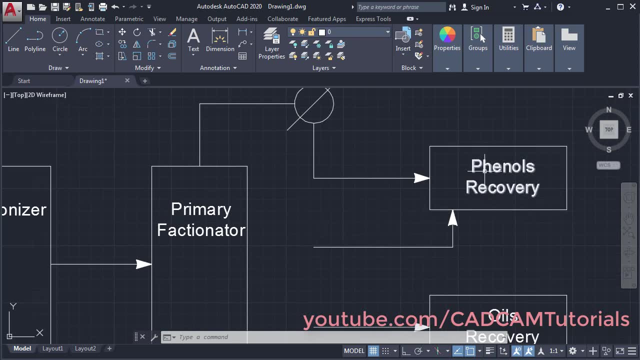 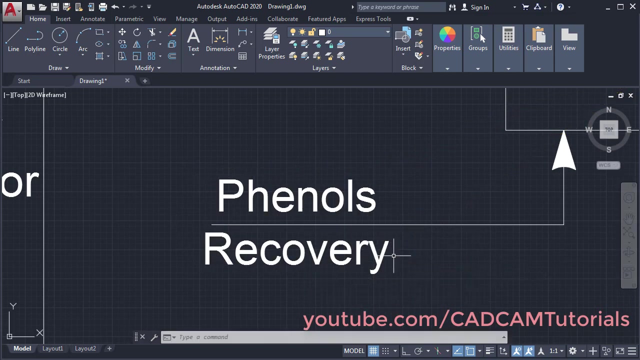 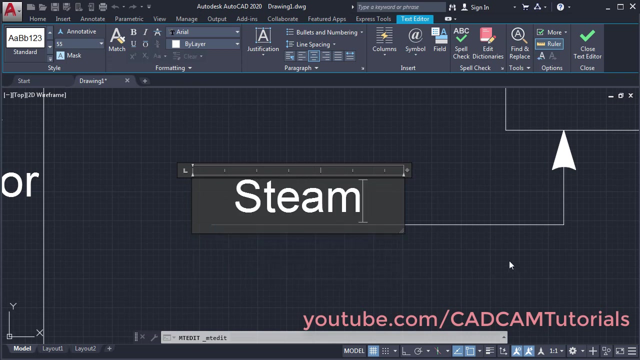 on the same point. take your cursor on this side and click enter. then we need to write their stream. for that we will copy this text. click on copy, select this text, enter. specify base point and zoom here and click enter. then double-click, select it and type their steam. click outside. 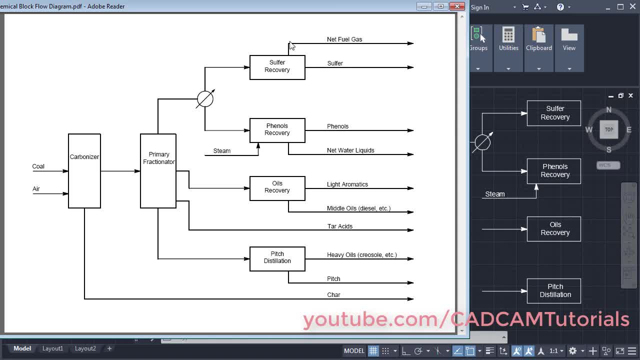 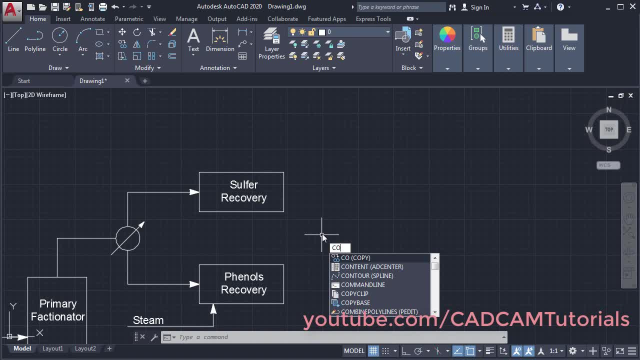 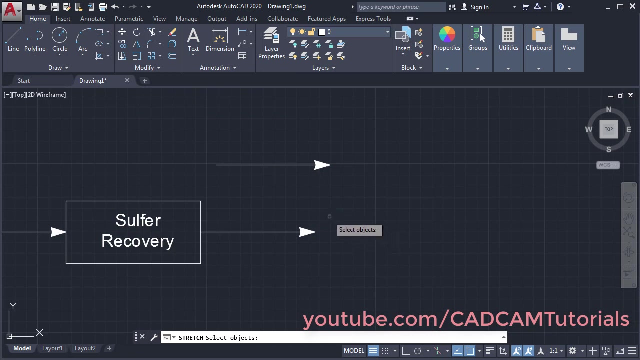 then we need these arrows going outside. you can also type C, O for copy: enter. select this object enter. specify this end point as base point and click on this midpoint and click here enter, then we will stretch it. click on stretch, then click here. take your cursor on the. 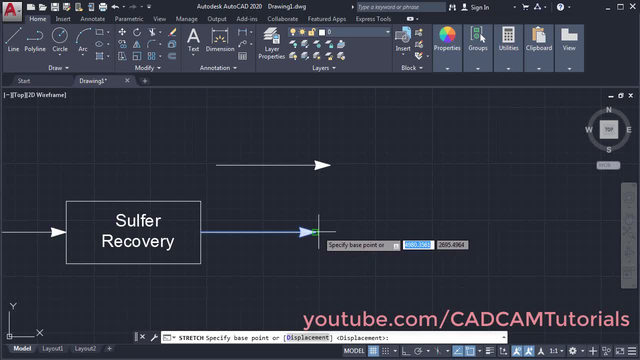 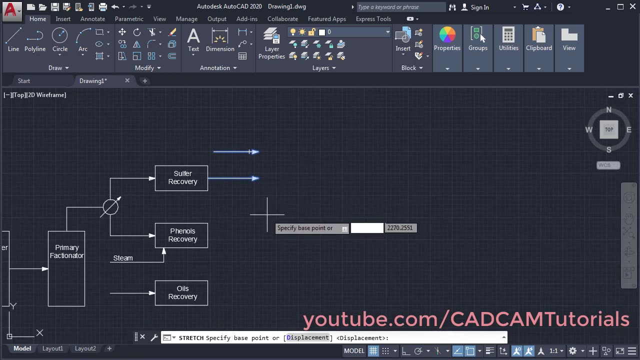 left side and click enter and click on this end point at first. we will match it. click, then press ENTER and again click in empty space. take your cursor on the left side, click enter, zoom minus. specify base point. take your cursor on the right side, make ortho on. 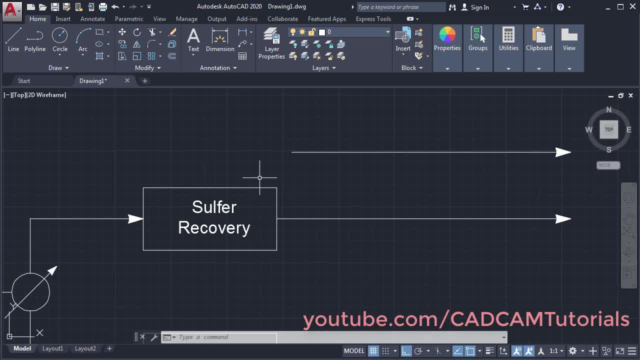 and click, then one line is needed here. click on line, take your cursor on the same point and take your cursor here and then in another line oraz at the end of line. click on line and clap my head, kiss into it away, then click, take it above, take your cursor to this end, point, track it. 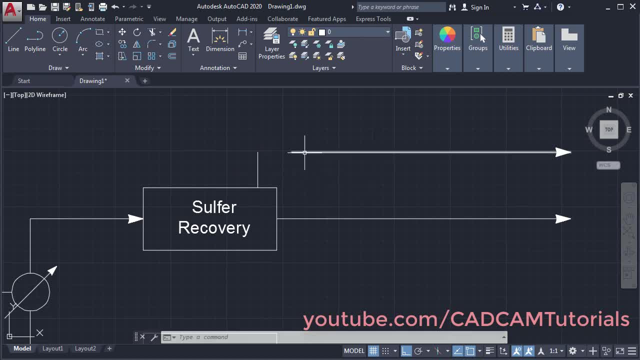 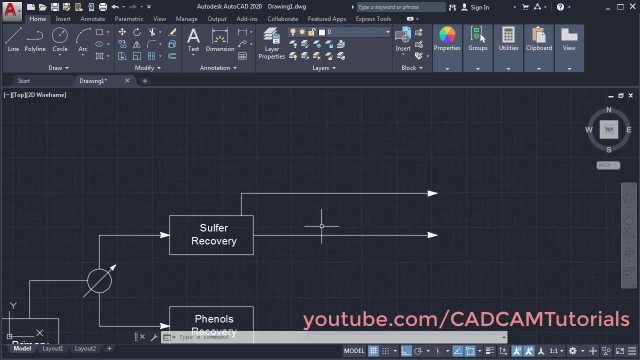 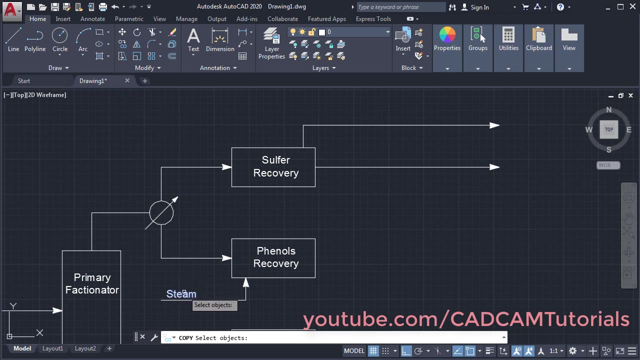 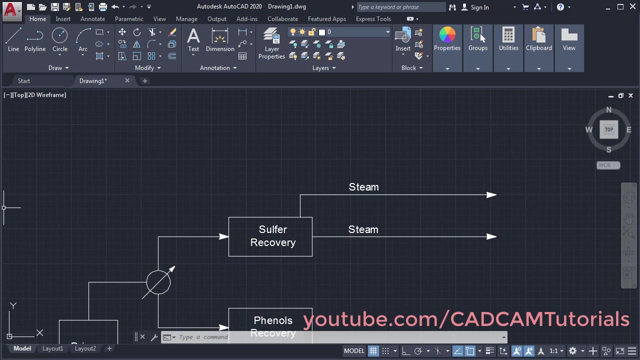 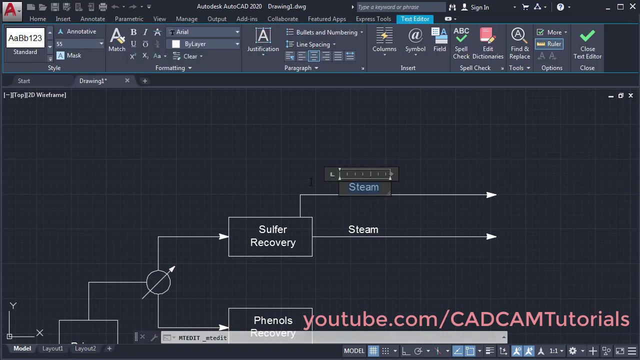 and click and enter and click on this line, click on this blue grip and click on this end point: escape. then we need text here again. click on copy, select this text, enter. specify base point here, make or throw off. and click here: enter. then it is net fail. gas and sulfur: double click. 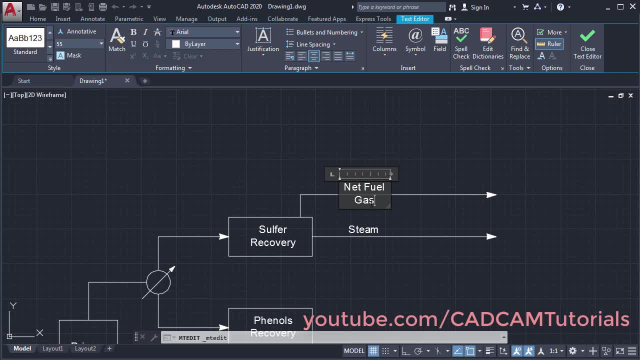 now here. it automatically became to line text. make it single line text. take your cursor on this inclined lines, then it will show arrow like this. then press and hold first mouse button and drag the mouse until it becomes single line text and release the mouse and click outside. 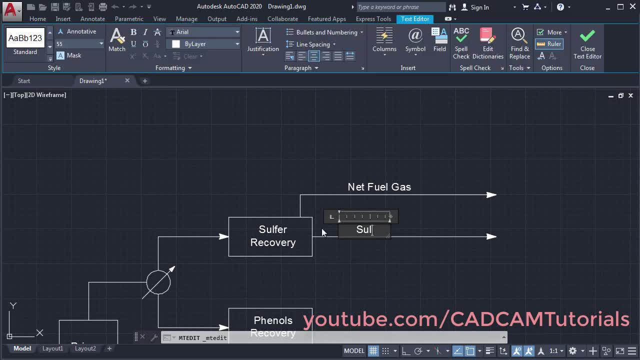 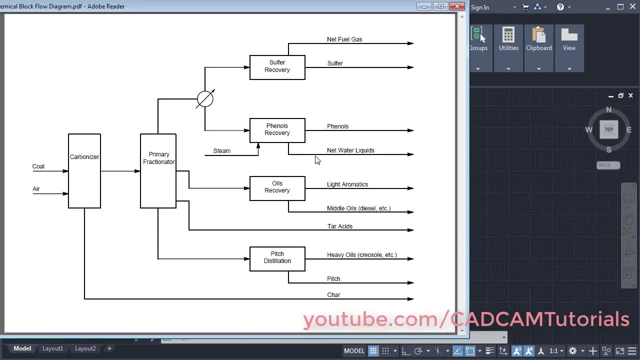 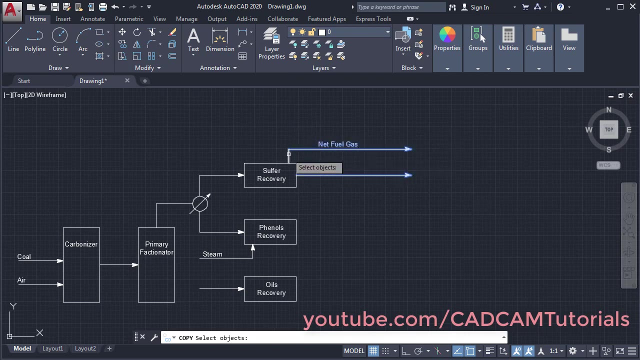 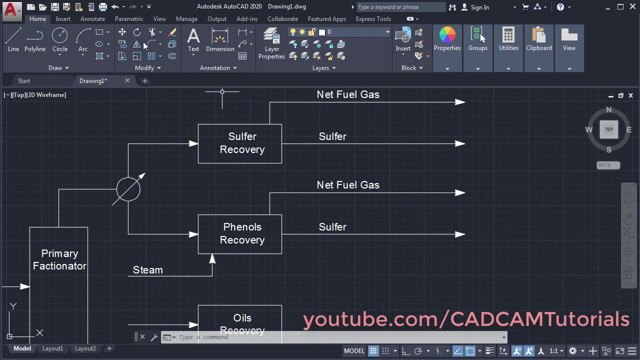 then double-click sulfur. click outside you. we will copy this below. click on copy. select this object. enter. then specify this endpoint as a base point and this end point as a second point: enter. we want this below. we will mirror this. click on mirror. select this object enter. 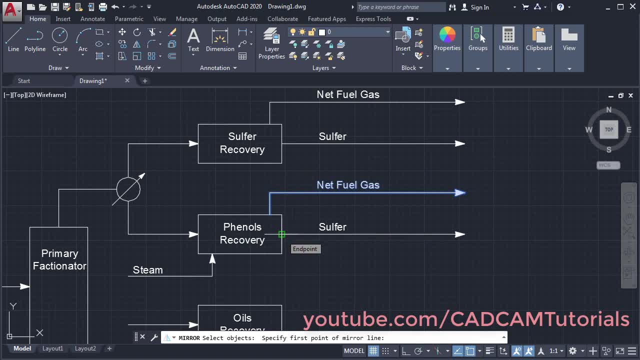 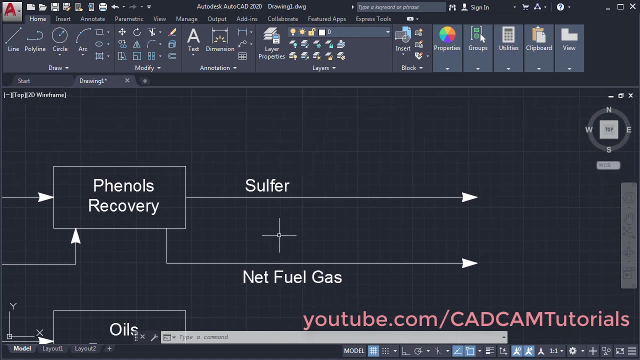 then worldКСП. then click on this end point for first point of mirror line. take your cursor on the right side. ensure that your line is straight. click then erase source objects. yes, then move this on upper side. click on move. select this object, enter. specify base point. take it above and 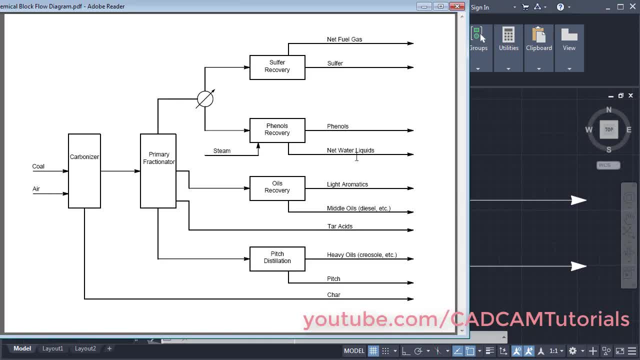 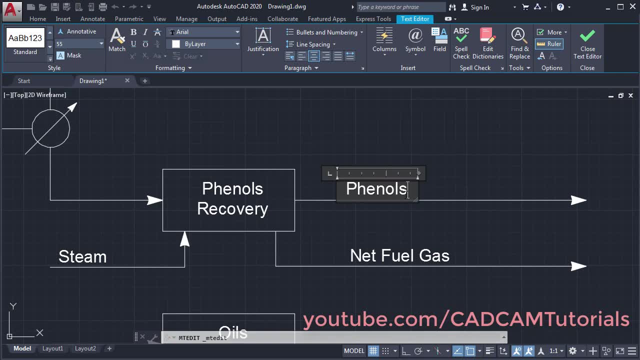 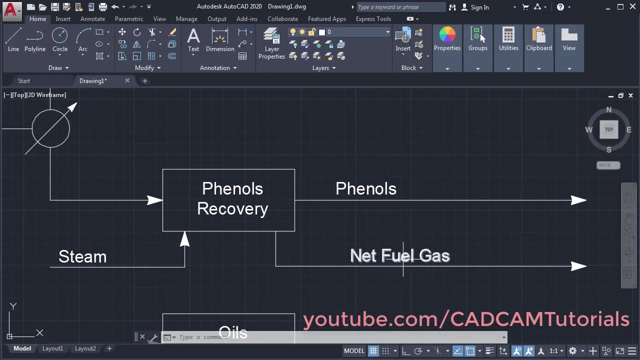 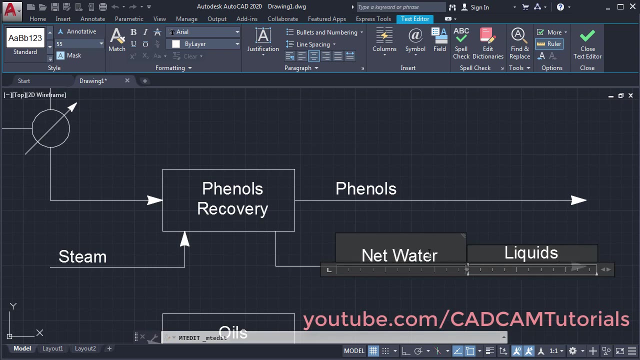 click then. this is phenols and net buttered liquids and this is required to be left aligned. click here on left, again double click then to bring it near. take your cursor on these three lines. once it shows inclined Iroq, press and side. hold first mouse button and take your cursor away, then select it and make it. 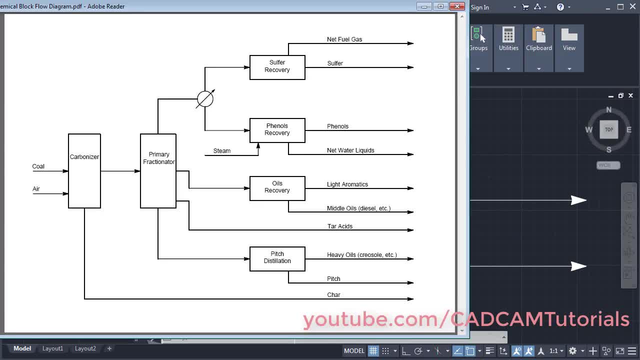 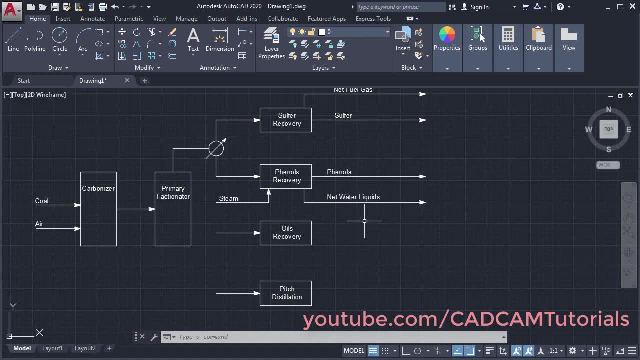 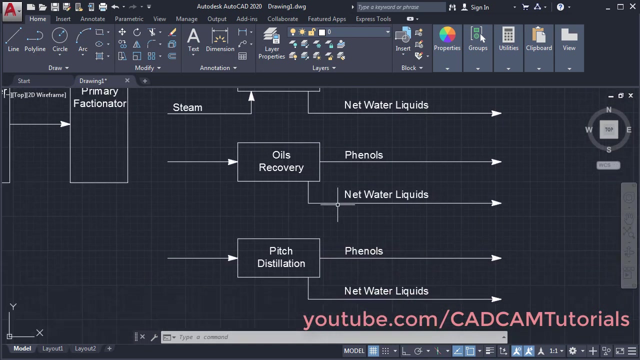 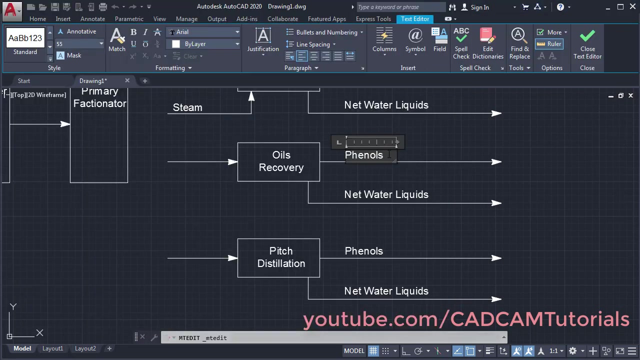 left align. click outside, then same is required below. we will copy it. you can also give copy command by typing for copy type C: O. enter then select this object. enter then specify this end point as base point and click here for second points. enter then light aromatics and middle oils double-click. 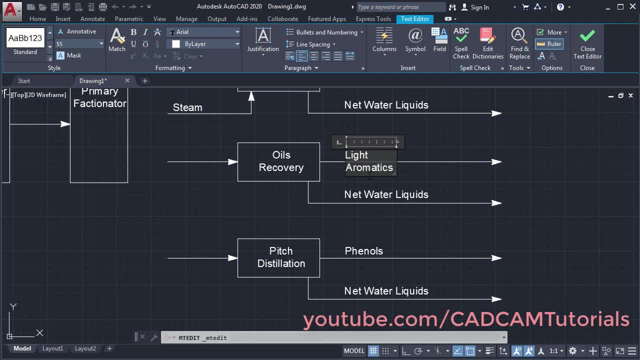 now it is shifted to second line. to bring it back in single line, take your cursor to this arrows, press and hold first mouse button and take your cursor away and release and click outside. you can also do it earlier rather than after arising of the problem, click outside. 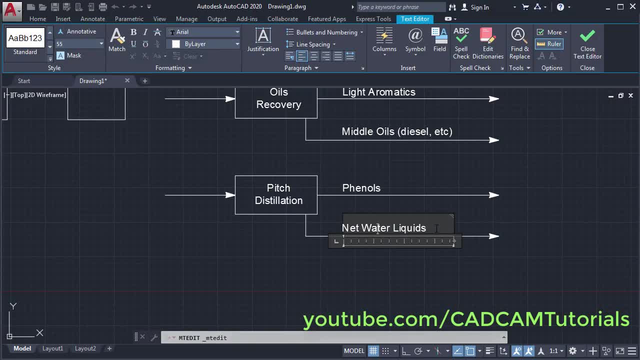 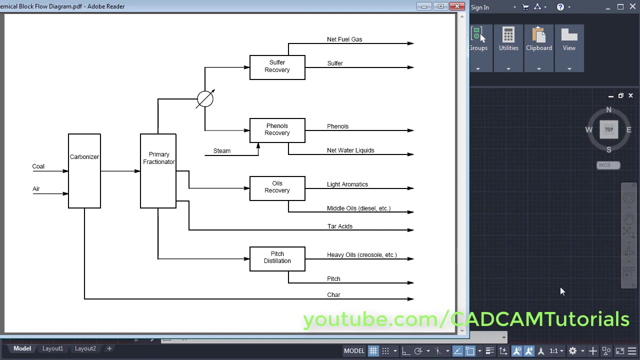 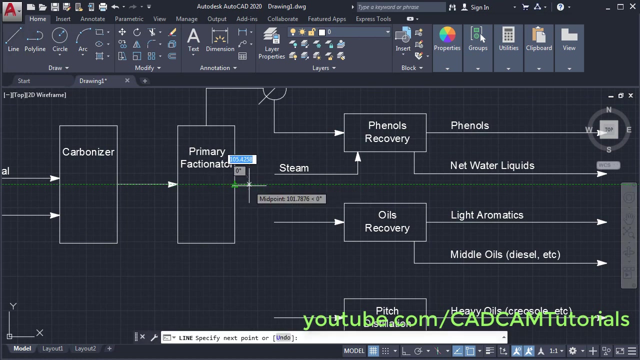 then heavy oils and pitch. double-click again. increase the size by holding first mouse button and dragging it. click outside. then we need to connect these lines. click on line, click on this midpoint, take your cursor on this side, take it below, drag this end point and click enter. then click on this line. click on this square. 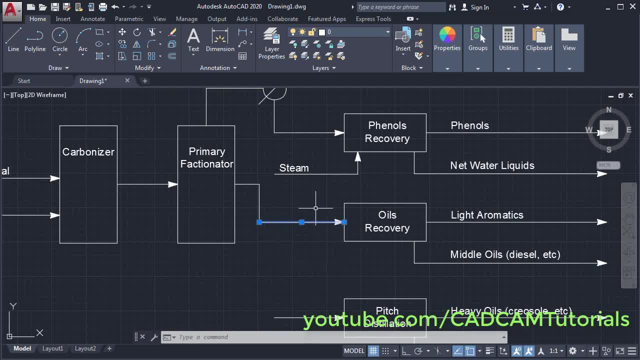 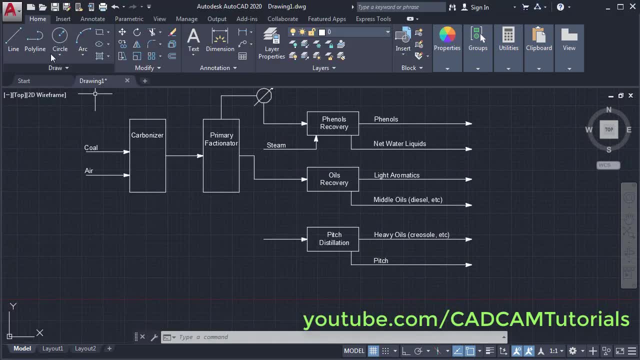 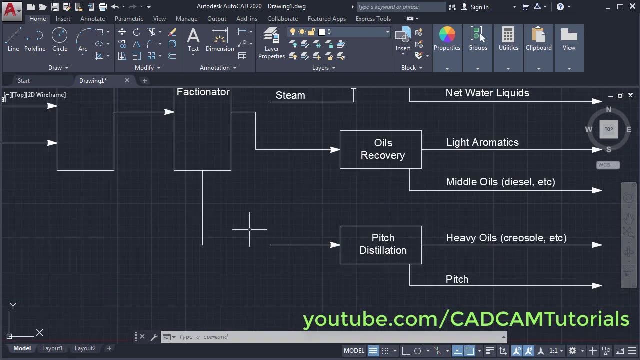 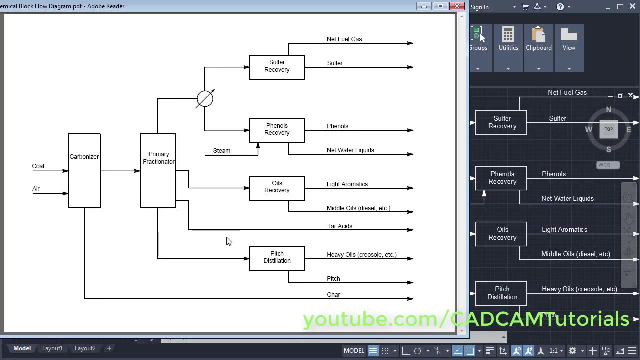 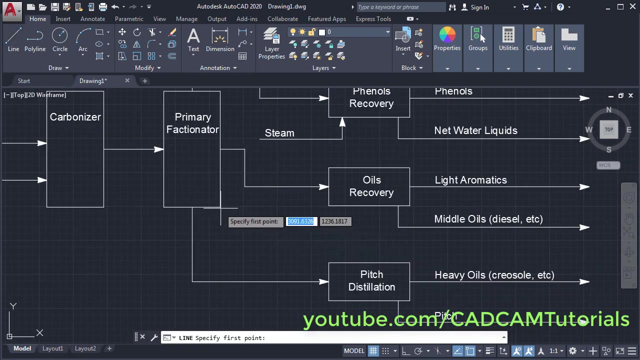 blue box and click on this end point. escape. then one connection from here: click on line. click on this midpoint, drag this end point, click enter. click on this line, click on this box, click escape. then this line, click on line, take your cursor to the same point. track that point, take your. 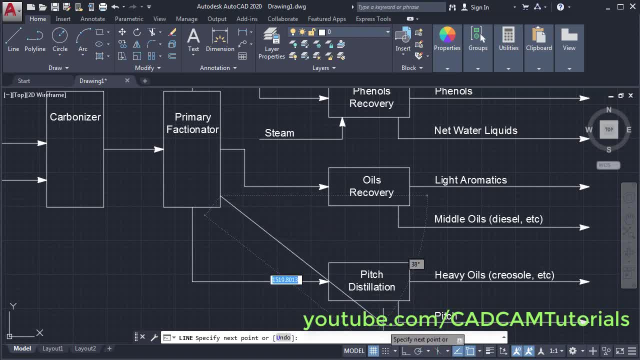 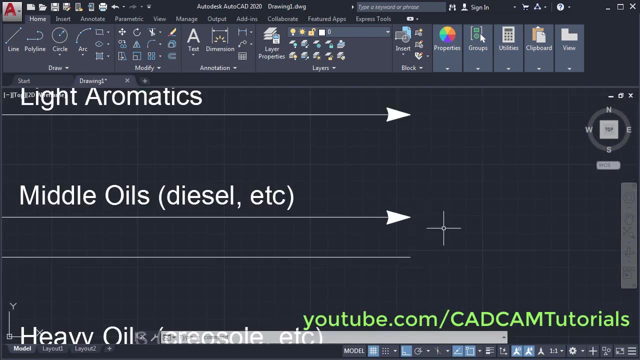 cursor above and click, then make ortho on, then track the same point, click, take it below and take it outside. track the same point and click and enter. then we will copy this arrow here. type co for copy: enter. select this object, enter. click on this end point and descend point: enter. 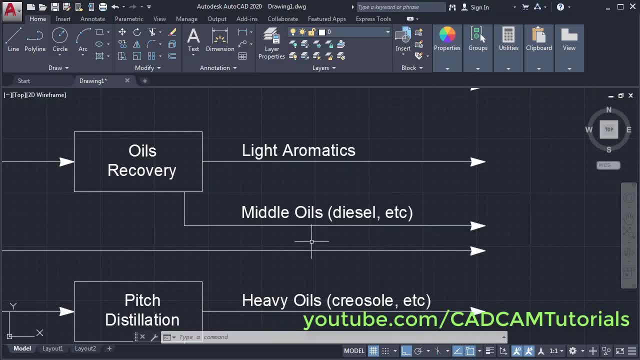 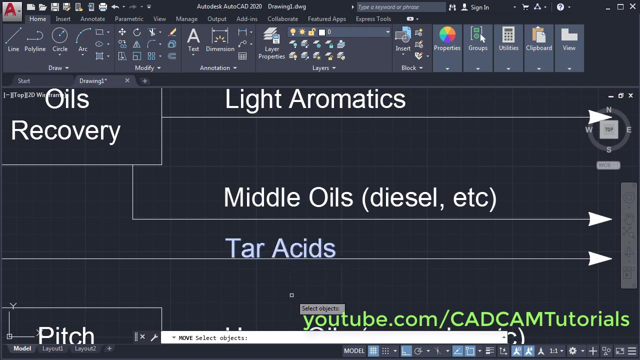 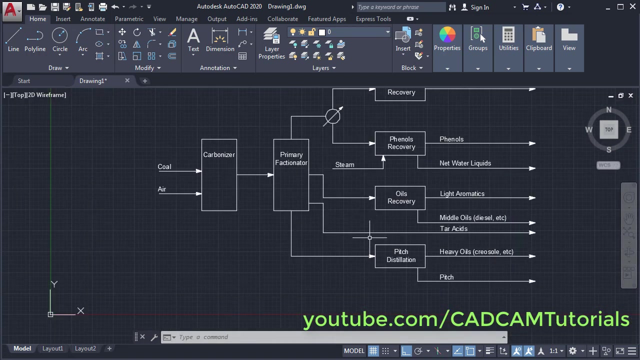 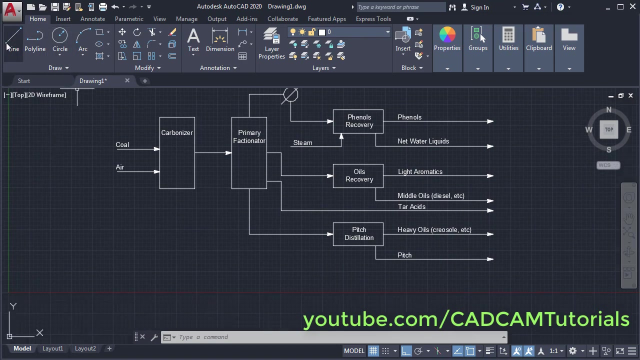 then text. copy this text: type: co: enter. copy this: enter specified base point. take it below and click enter double click. click outside. take it above. type M for moveow. select this text: enter. specify base point here. take your cursor above and click then this: one. click on line. click on this midpoint. take your cursor below, click. take it on this side track. 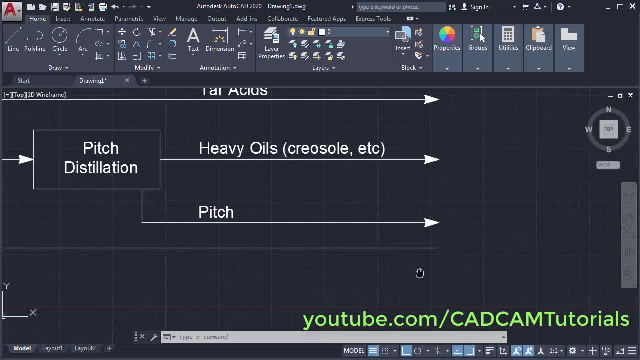 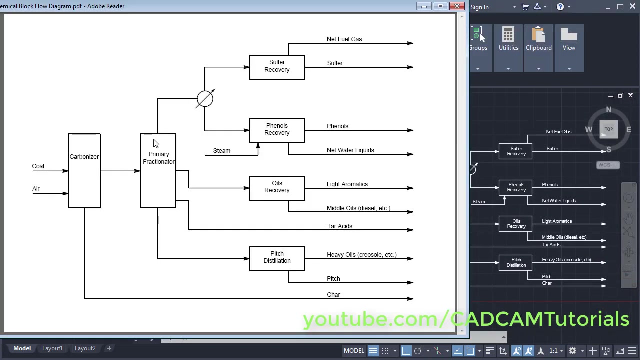 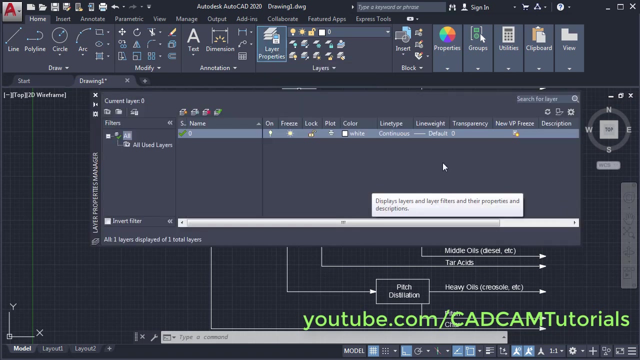 this end point, click enter, then copy this text. an arrow click on copy. click this text and this arrow enter. specify this point at this end point and click enter and double-click. click outside and assign this thickness for that. click on this layer properties. click here on default and select this thickness. okay, close this dialog box then to show the 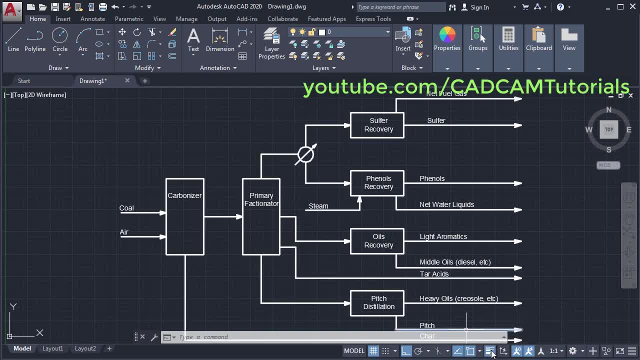 thickness. click here on show head line width. the thickness is shown, so this drawing is ready. in the next tutorial we will create, next chemical engineering time, and we will also continue our autocad basic tutorials. and we will also continue our autocad basic tutorials and we will also continue our autocad basic tutorials and we will 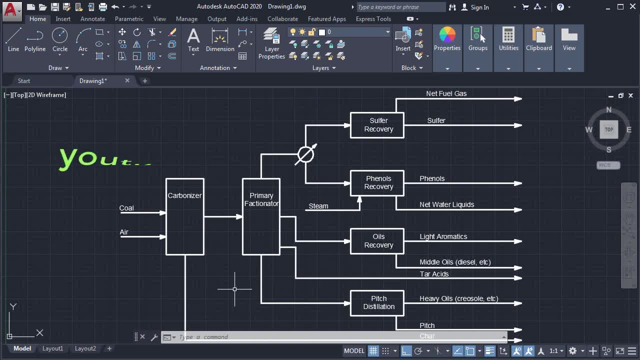 all. see you in the next video, Thank you. also saw all exercises on those tutorials and we will also continue our civil electrical and interior design tutorials. so thanks for watching. we will stop here.